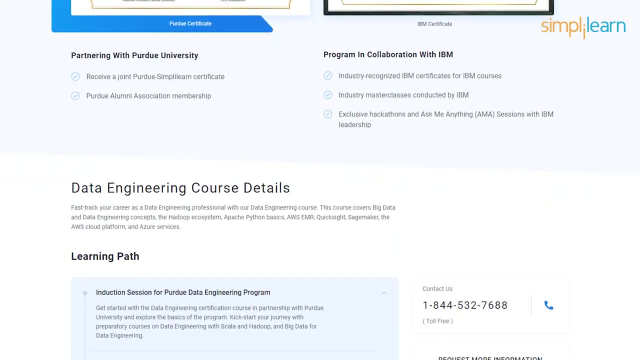 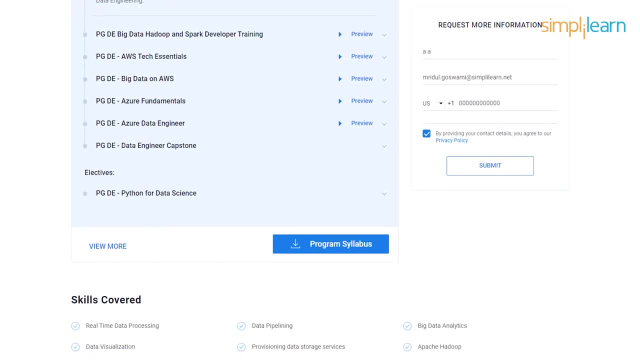 program utilizes various learning methods, such as live sessions, industry projects, IBM hackathons and ask-me-anything sessions to provide a comprehensive and practical learning experience. So what are you waiting for? Enroll now in the postgraduate program to kickstart your 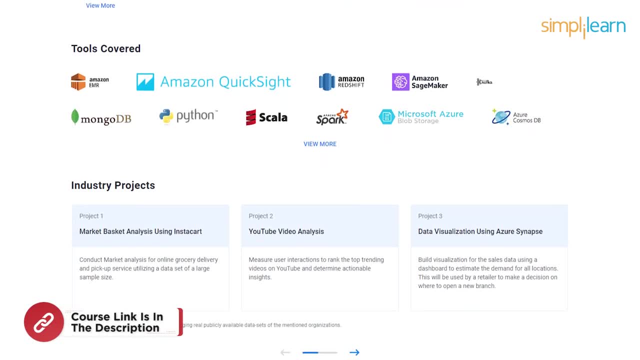 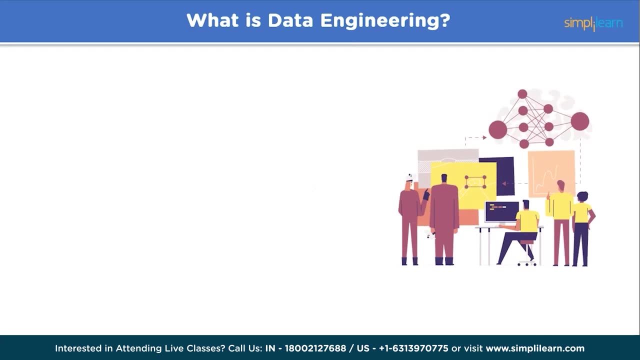 journey in data engineering. The course link is added in the description box below. Make sure to check that out. So, without any further ado, let's get started with today's topic. Firstly, let us understand what is data engineering. Data engineering involves building pipelines. 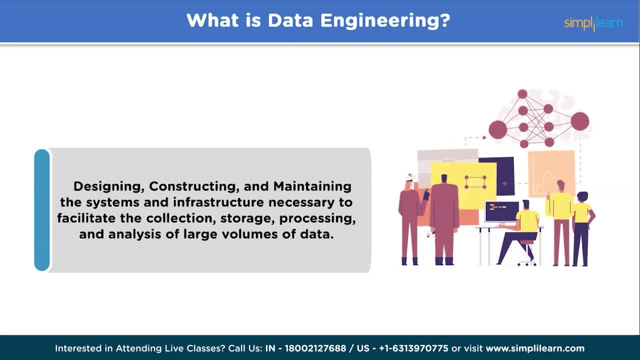 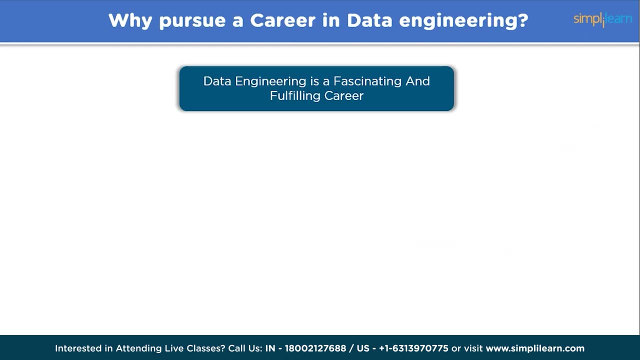 that extract, transform and analyze large-scale data to provide valuable insights about a business operation. By leveraging these insights, organizations can create a cooperative edge, improve efficiency and improve productivity. Now the main question is: why pursue a career in data engineering? Well, data engineering. 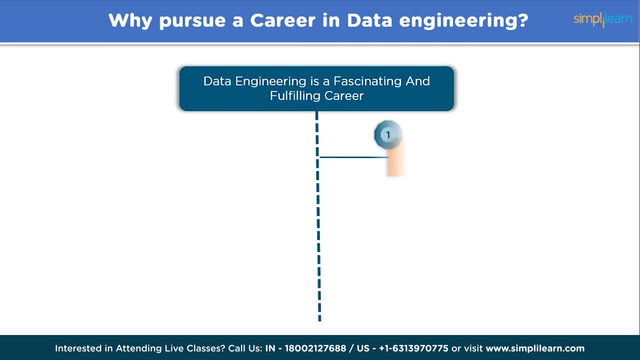 can be a fascinating and fulfilling career. The reason for learning data engineering nowadays is because of its high demand and growing landscape in our current business. technological trends Like the demand for data engineers is constantly increasing as organizations recognize the value of data-driven decision making. Now companies across various industries 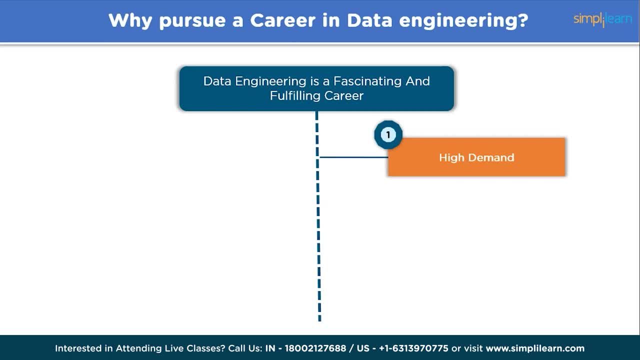 are investing heavily in data infrastructure, analytics and machine learning, creating a high demand for skilled data engineers. Secondly, diverse industries. Now there are a variety of job opportunities in the field of data engineering. Data engineering offers a wide range of job opportunities in which you can work in various industries, such as. 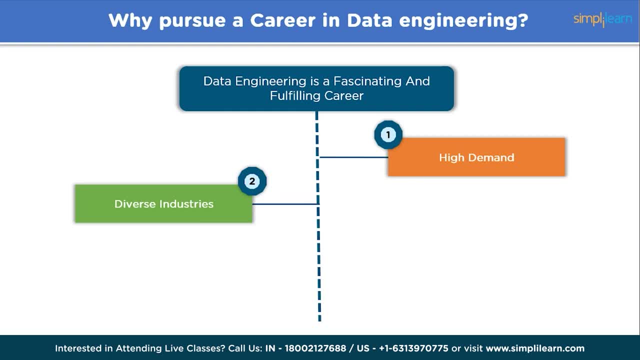 technology, finance, health care, e-commerce and much more. Additionally, you can choose to work up in large corporations, start-ups, consulting firms or even as a freelance data engineer. Next competitive salary: To get the competitive salary, you can work in two. 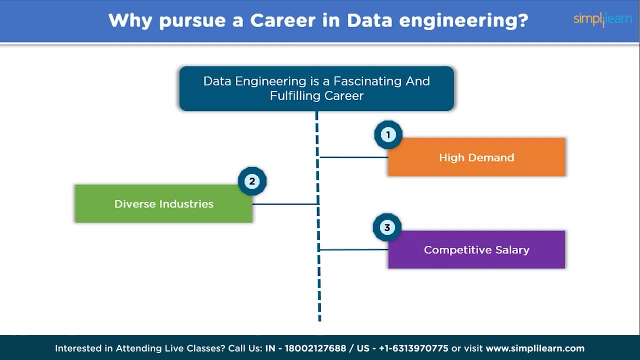 sectors. One is among the major companies and the second is in the industry, which is Now data engineer. skills are highly valued in the job market nowadays, and a competitive compensation is what makes a part for a data engineer in the market. This demand often translate into competitive compensation packages and opportunities for 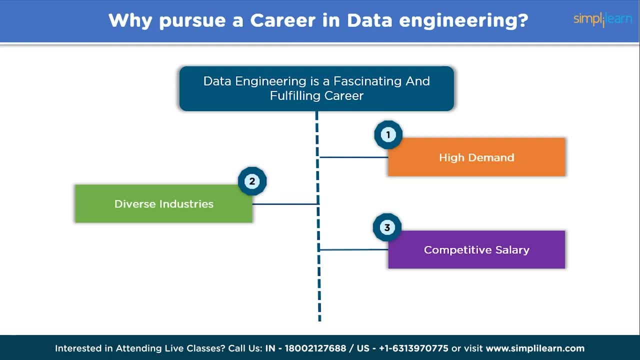 career growth. As you gain experience and expertise, you can attain leadership roles with handsome salaries. And, finally, problem solving and continuous learning. Now, data engineering is a field that constantly evolves. New technologies, tools and frameworks emerge regularly, offering opportunities for continuous learning and growth. 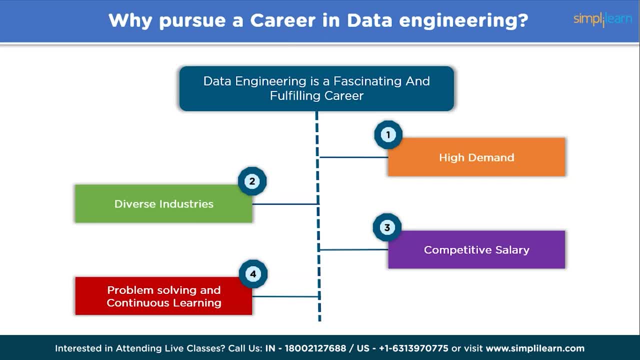 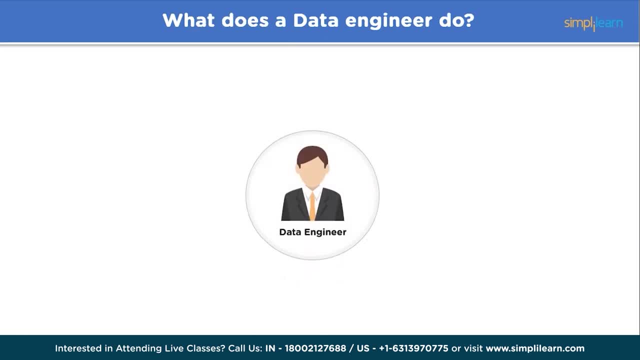 As a data engineer, you can stay at the forefront of technological advancements, acquire new skills and expand your knowledge to adapt to changing industry trends. Now let us understand. what does a data engineer do? Now? a data engineer is responsible for designing, constructing and maintaining the infrastructure. 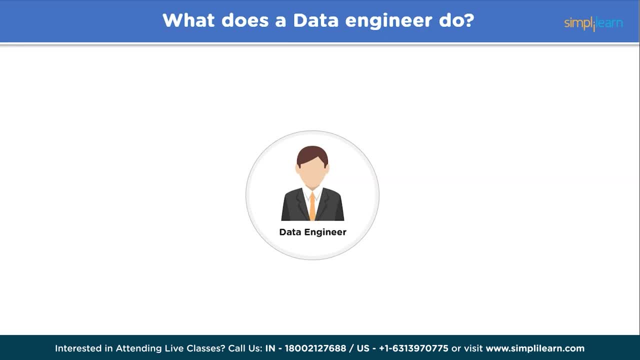 and systems required for the efficient and reliable handling of large volumes of data. So, on a daily basis, a data engineer involves in many aspects, Activities such as data pipeline development. Now, data engineers build robust and scalable data pipelines that extract, transform and load data from various sources into storage and processing systems, ensuring data quality. 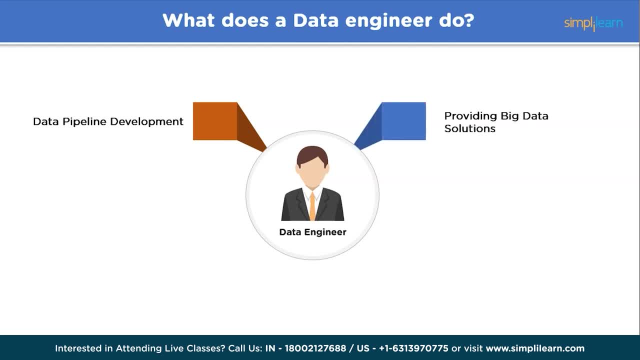 integrity and efficient data movement. Providing big data solutions: Now data engineers work with big data technologies such as Apache, Hadoop, to handle large volumes of data, parallel processing and distributed computing. Data warehousing and integration: Now Data engineers design and implement data warehouses, which are centralized repositories that store 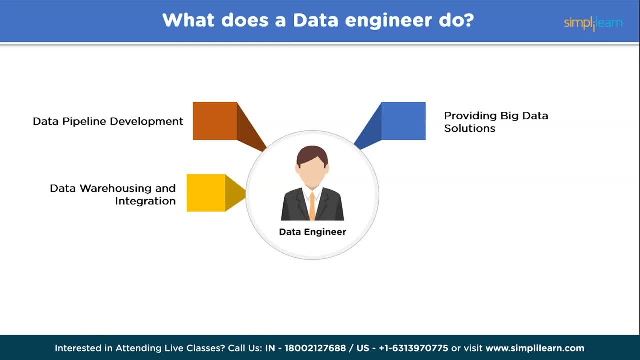 structured, semi-structured and unstructured data. Data engineers integrate data from multiple sources, including database, API and external systems, in order to consolidate and reconcile data from various sources, ensuring data consistency and coherence, Performance and optimization. Now data engineers optimize data processing workflows, database queries and system performance. 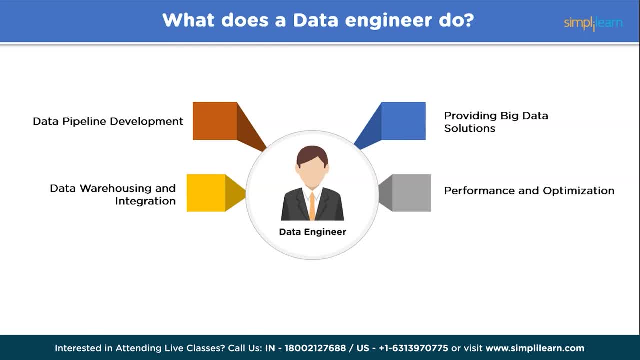 to minimize latency, improve efficiency and efficiency. Now data engineers work with big data technologies such as Apache, Hadoop, to handle large volumes of data. parallel processing and distributed computing Then enhance overall system performance. MySQL and Oracle, which provide an extensive collection of database management Natomiast. 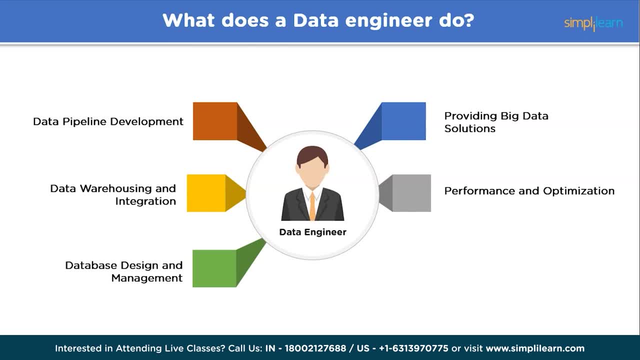 binaural system performance. database design and management: Now database engineer design, create and maintain databases, selecting appropriate database management systems like MySQL, Oracle and others, ensuring efficient data organization, indexing and query performance. And, finally, monitoring and maintenance: Now data engineers monitor data pipelines, databases and system, help to identify and 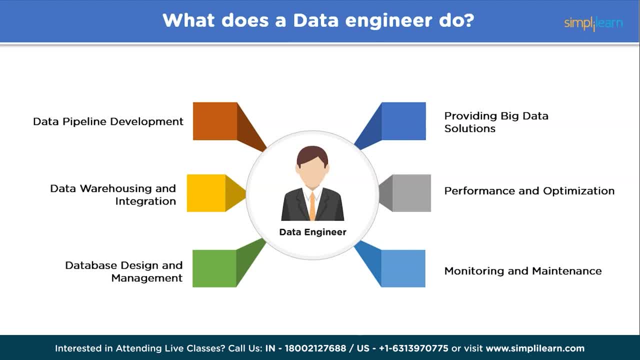 resolve issues promptly. They perform routine maintenance, Backup and backup, backup and maintenance, backups and upgrades to ensure system reliability and stability. So these are some of the day-to-day responsibilities of a data engineer. Now let us now move ahead and discuss some of the data engineer skill set. 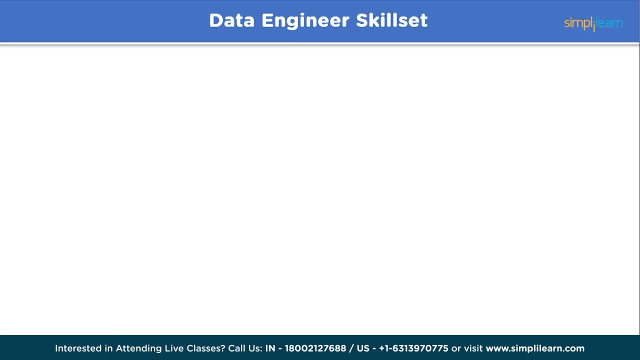 Now, becoming a data engineer requires a multi-disciplinary skill set: branding, software engineering, data management, big data and cloud computing expertise. Firstly, having a good knowledge on database knowledge. Now, data engineers are well versed in working with relational databases like MySQL, Oracle. 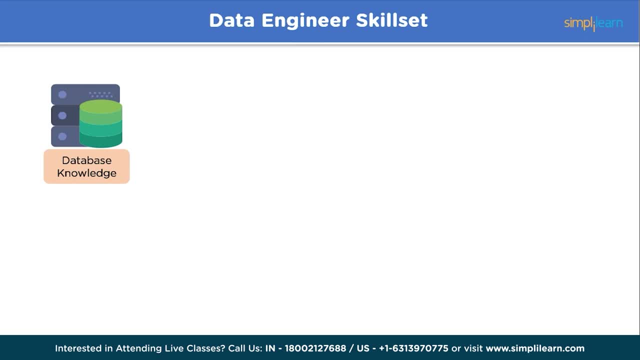 PostgreSQL and even non-relational databases like MongoDB, Cassandra and Redis. They should have a strong understanding of database design, schema modeling, indexing and query optimization. Statistics Now, just like the field of data science and data analytics. having a good knowledge on statistics for data engineers can set them. 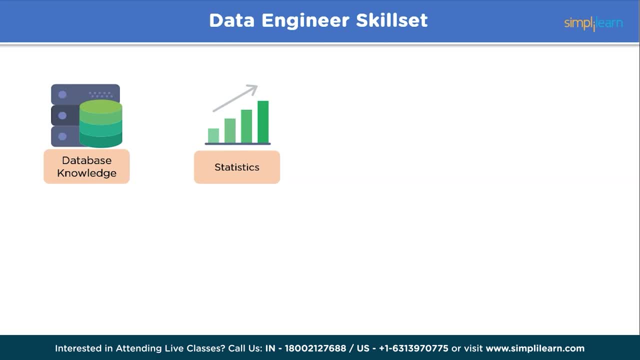 apart from the rest. So having a good analytical skills on mathematical models and statistics and probability can help you stand out in the market. Programming Tools. Transparency in programming language is crucial for data engineers. They commonly work with languages such as Python, Java, Scala to develop data pipelines. 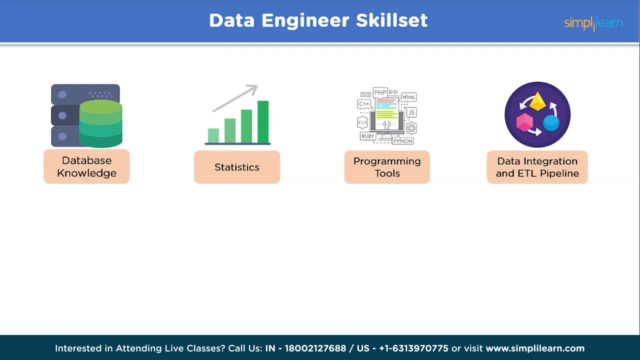 automate processes and perform data manipulation tasks: Data Integration and ETL Pipeline. Now, understanding the concepts and techniques related to data warehousing is important for data engineers. ETL pipeline, which is a part of data warehousing, is responsible for extracting data from various 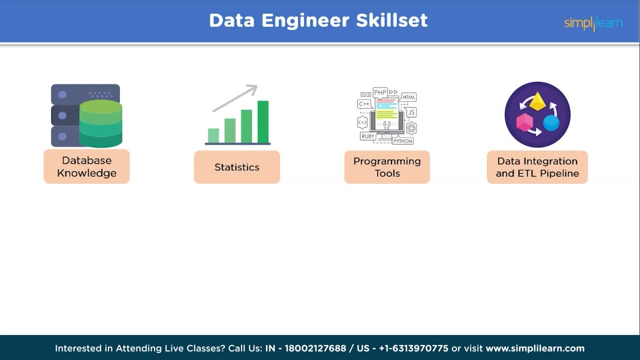 sources, transforming it into a usable format and loading into data warehouses- Machine Learning. Now, although data warehousing is a very complex and complex process, data warehousing can be done in multiple ways. Data engineers don't have much reliance on machine learning, but having a good knowledge, 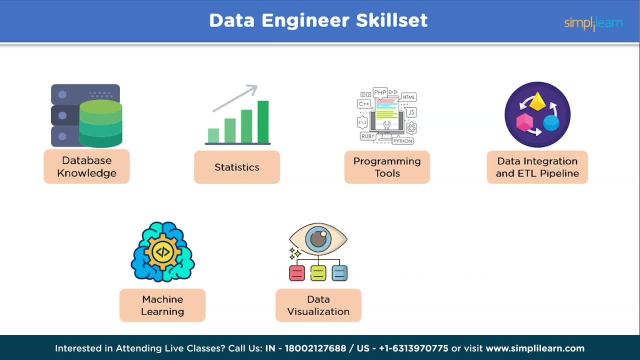 on machine learning can also provide you an edge over the others. Having a good knowledge and skills on data visualization tools like Tableau, Power BI and QlikView can help you gain a competitive advantage in the job market as well. Big Data and Cloud Computing. 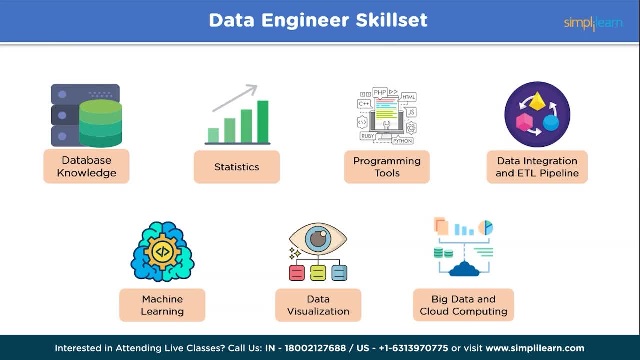 Data engineers work with large-scale data processing frameworks and technologies, and having a good knowledge on big data tools like Apache, Hadoop, Microsoft Office Word, Microsoft Office Word and Google Docs can help you gain a competitive advantage in the job market as well. 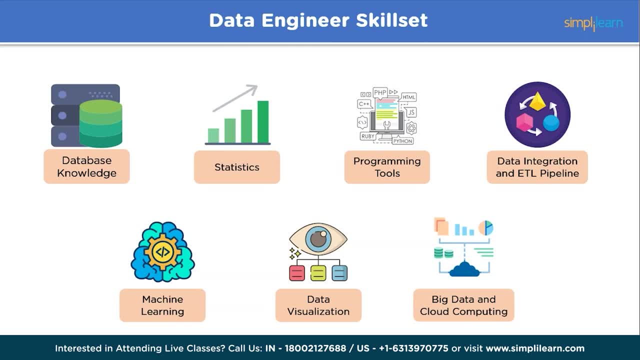 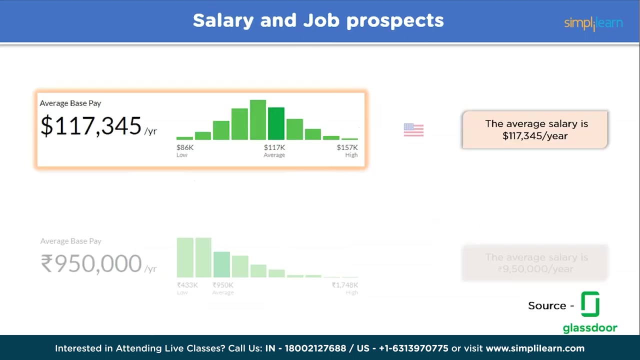 In addition, data engineers also often work on cloud platforms like Amazon Web Services, Microsoft Azure and GCP for building and deploying data solutions. All these are some of the main skills that a data engineer should possess in order to thrive in today's technological domain. 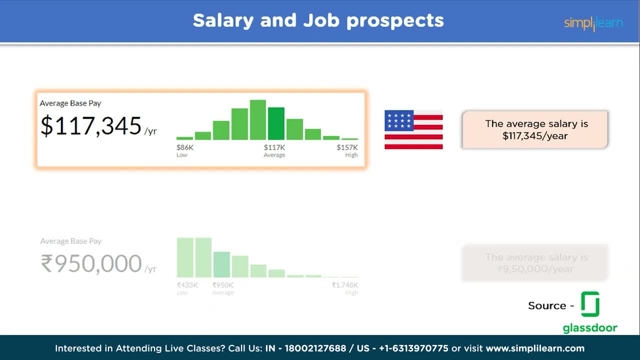 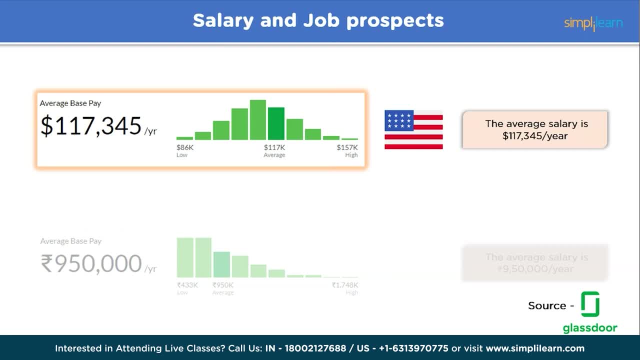 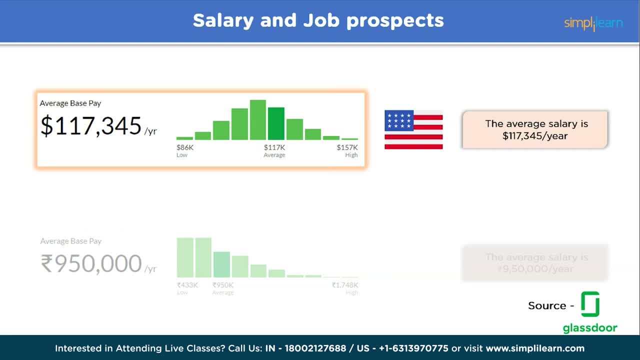 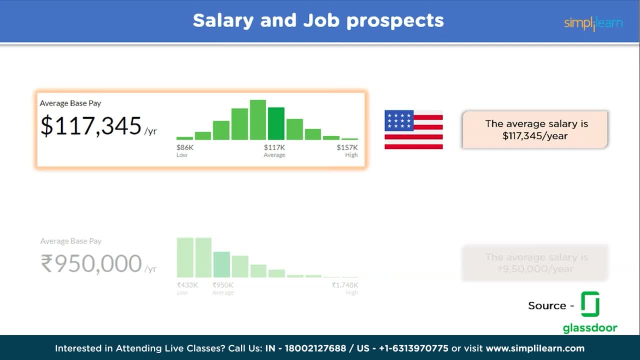 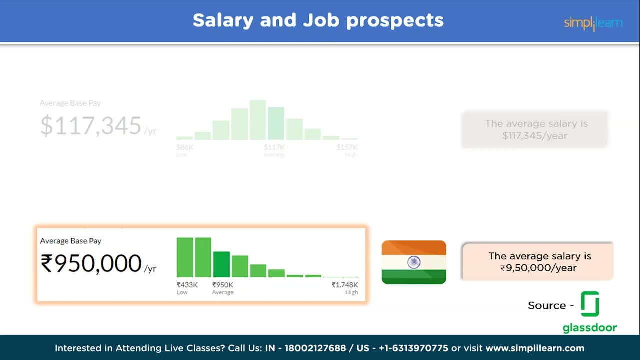 Salary and Job Prospects of a Data Engineer. Salary and Job Prospects of a Data Engineer: thousand dollars per year. similarly, in india, if you talk about the average salary, it is around 9.5 lakh per year and can go high- as high as 17 lakhs per year. so as companies invest heavily in data. 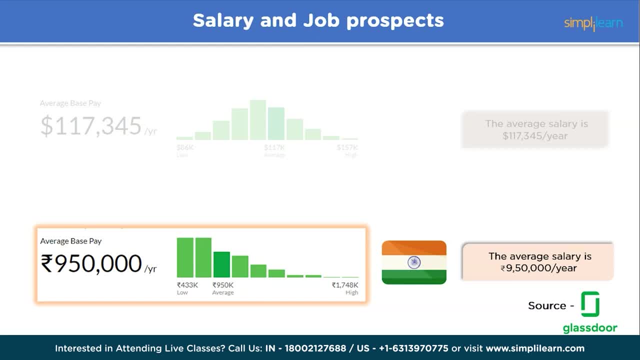 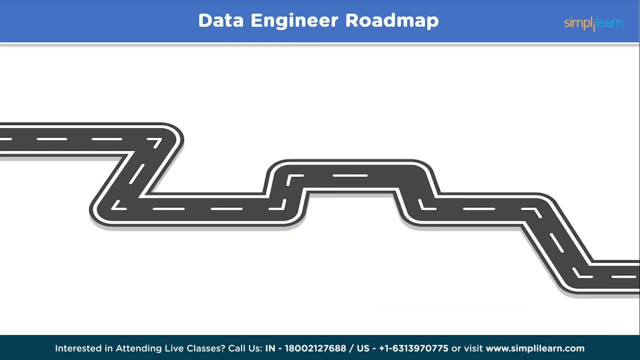 driven initiatives. they are willing to pay a premium for skilled data engineering professionals who can help them harness the power of their data in today's digital era. now, becoming a data engineer doesn't happen overnight. you need to have a blend of technical skills, practical experience on various tools and technologies in order to become a data engineer. so let us now directly. 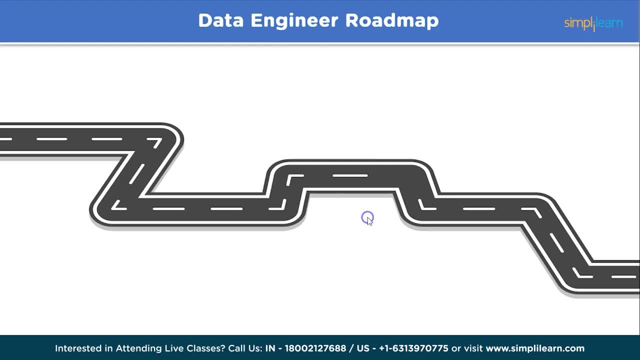 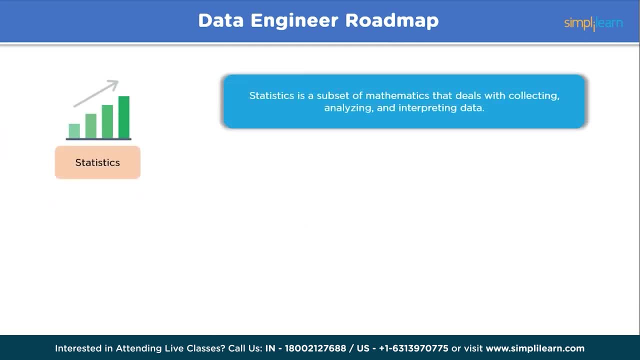 dwell into the roadmap on how to become a data engineer. firstly, have a strong foundational knowledge. now develop a strong foundation in mathematics and statistics, just like data science and data analytics do. now, data engineering heavily relies on mathematical, statistical concepts, so and various statistical tools. so begin by strengthening your knowledge in areas such. 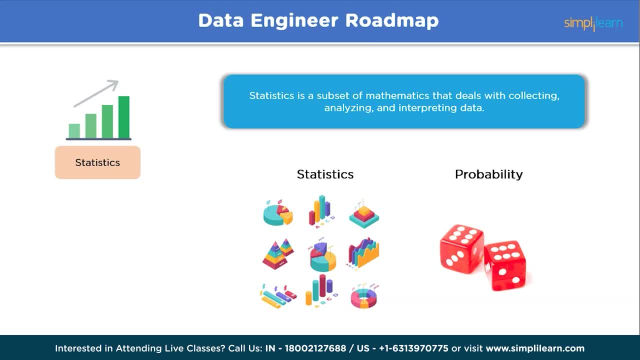 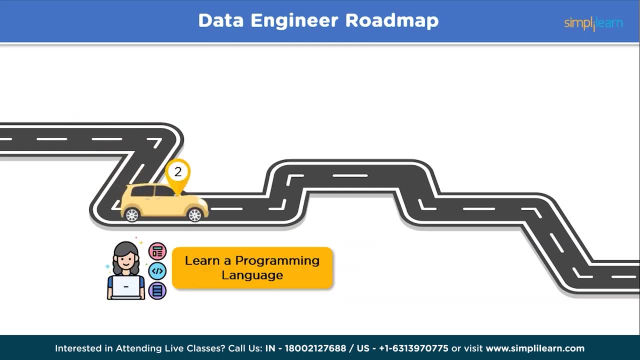 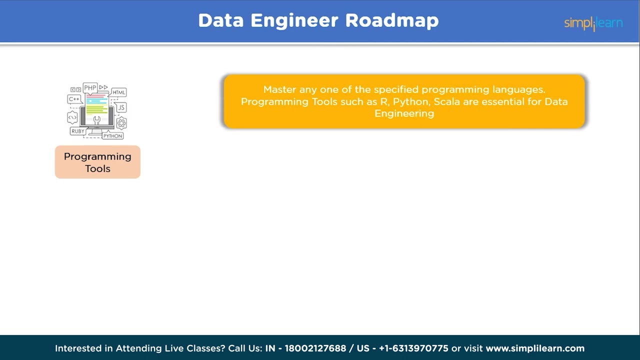 as linear algebra calculus, probability theory and statistical analysis. now moving ahead, you need to have a strong foundation on any of our programming languages now. to embark on a journey as a data engineer in 2023, mastering a programming language is paramount now. python stands out as an ideal choice to begin your programming journey in this field. 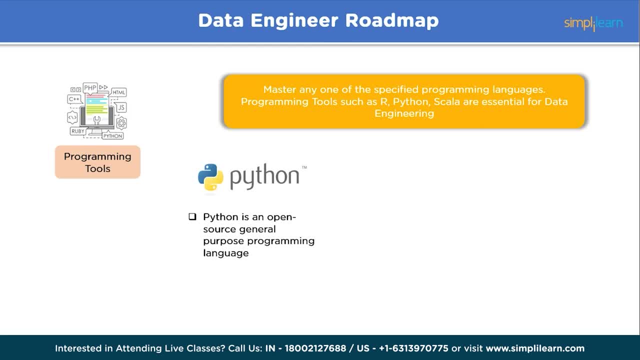 providing a solid foundation and structured thinking. python is widely regarded as one of the most suitable languages for data engineering. its user-friendly syntax and readability makes it easy to learn and understand. it offers an extensive range of libraries and frameworks, such as pandas, numpy and scipy, in order to efficiently handle and transform data. 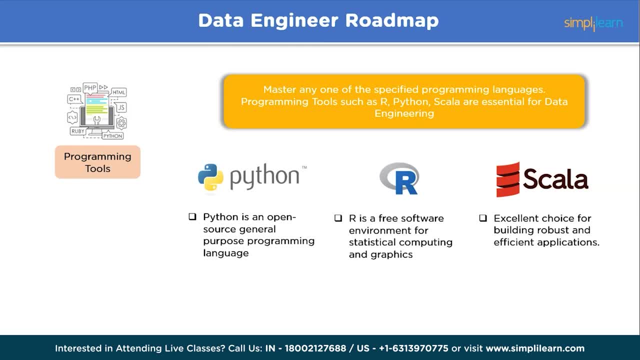 in addition, you can also master languages like r and scala, which are more popular these days for data engineers moving ahead. have an in-depth knowledge on databases. you can also master languages like r and scala, which are more popular these days for data engineers moving ahead. have an in-depth knowledge on databases. 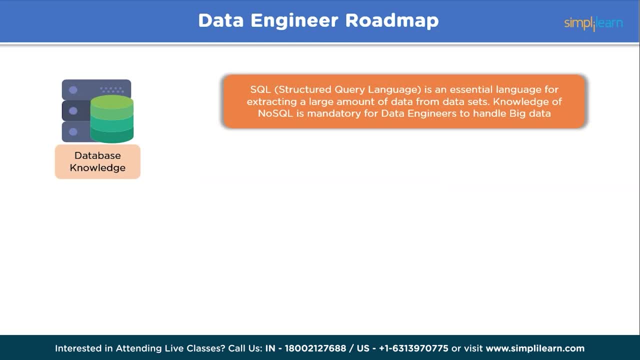 now as a data engineer. working with database systems is a fundamental aspect of your role, as you play a vital role in handling large data sets efficiently. now, with a plethora of dbms options available, it's important to note that you don't need to be expert in all of them. the choice of 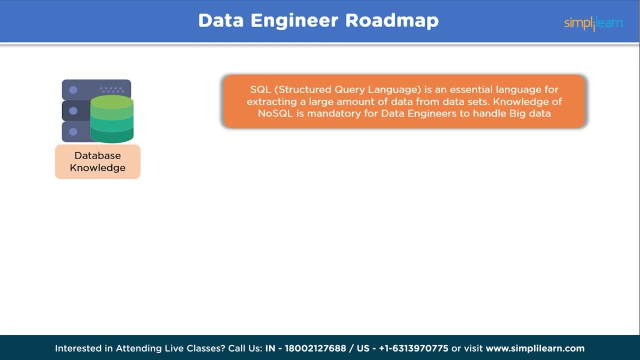 dbms often depends on the space requirements and preferences of the company you work for, as well as your own preferences and expertise. now, rdbms such as oracle, microsoft, sql server, mysql, are widely adopted for managing structured data. they provide a well-defined schema, transactional support and robust querying capabilities. 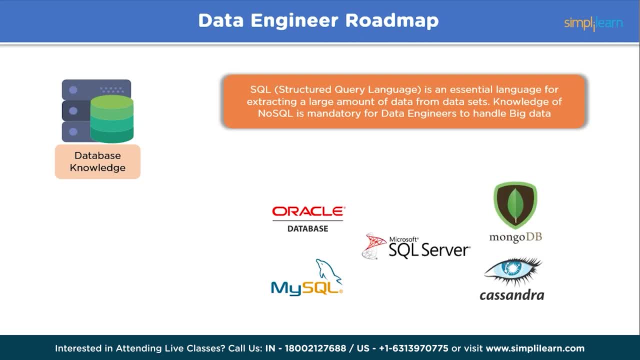 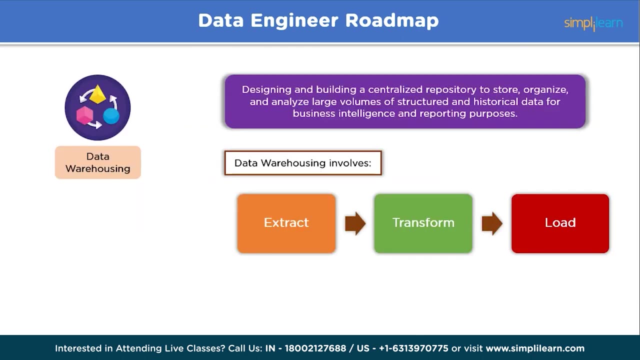 no sql databases like mongodb, cassandra are designed to handle unstructured or semi-structured data. they offer flexibility in data modeling, horizontal scalability and high performance for specific use cases. well moving ahead data warehousing and etl pipelines. now data engineers specialize in designing and building data infrastructures, including 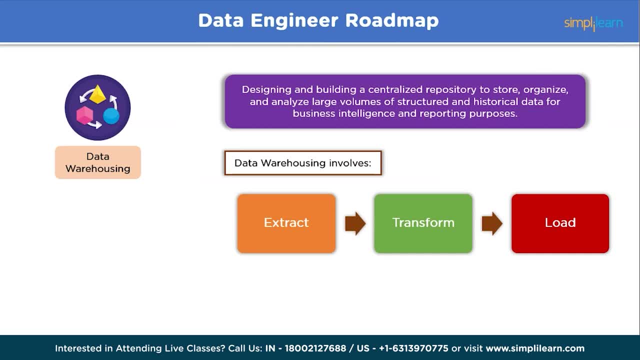 data pipelines and data warehouses. they are responsible for efficiently collecting, transforming and storing data from various sources. now, ETL stands for extract, transform and load, and it refers to the process of extracting data from various sources, transforming it into a consistent and structured format. now, ETL plays a crucial role in data warehousing by enabling 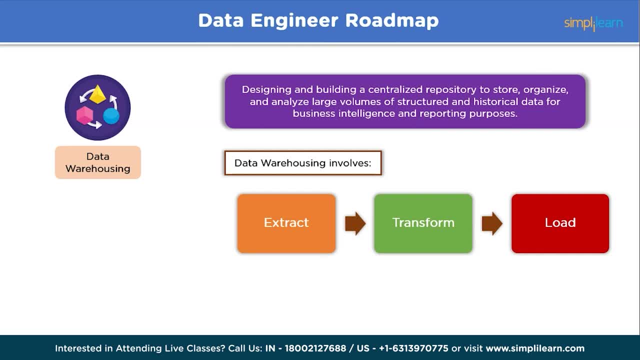 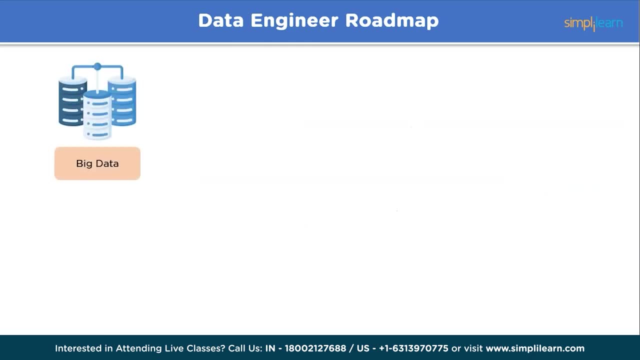 organizations to integrate and consolidate data from diverse sources into a central repository. well, moving ahead, you need to master big data tools now. handling large data sets is a common requirement for data engineers and to accomplish this effectively, you often need to work with big data tools now. these tools complement their knowledge of cloud computing as data engineers. 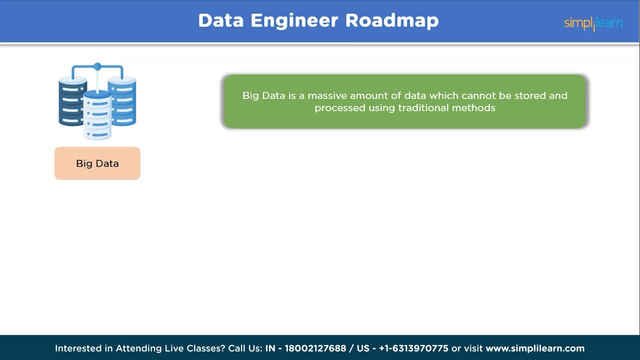 frequently implement code that can handle and process large data sets in a cloud environment. therefore, having experience with tools such as apache spark, which is a powerful distributed processing framework that enables fast and scalable data processing and data processing, it provides a unified and flexible platform for batch processing. real-time streaming machine. 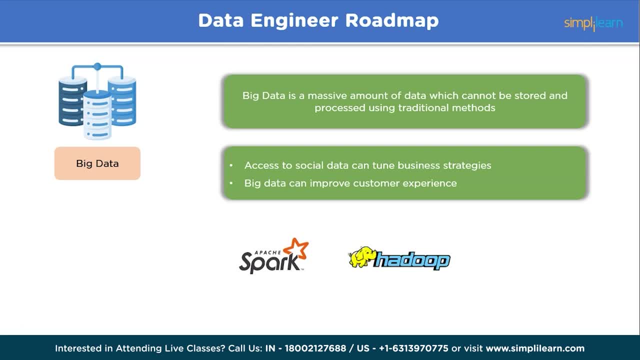 learning and graph processing, and apache hadoop, which is an open source framework for distributed storage and processing of large data sets across cluster of computers. it includes the hadoop distributed file system, or in short known as HDFS, for scalable storage, and map reduced programming model for distribution processing. and, finally, apache kafka, which is an open source. 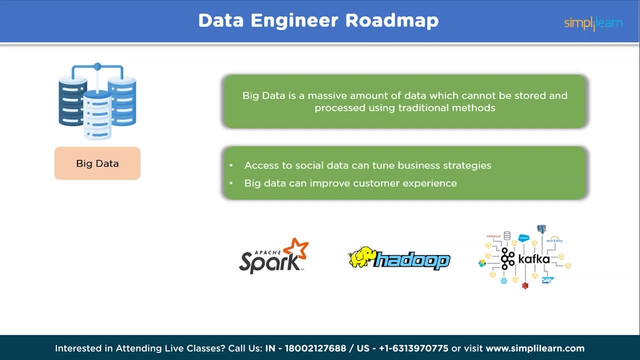 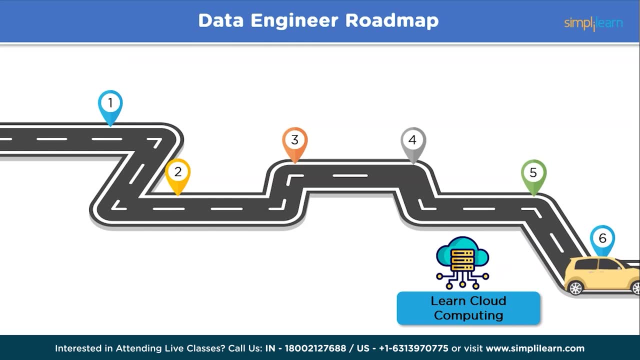 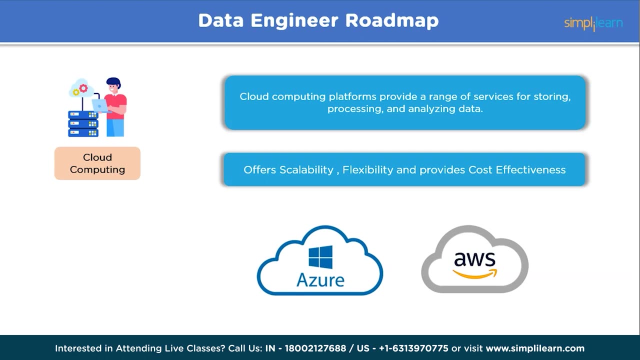 distributed streaming platform developed by the apache software foundation. it is used to handle real-time high throughput and fault or in streaming data. and finally, learning cloud computing. well, cloud computing has revolutionized the way businesses store, process and manage their data, leading to a growing demand for engineers skilled in cloud computing tools and platforms. now the three. 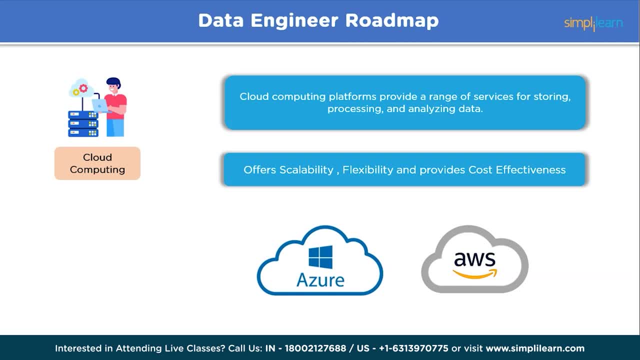 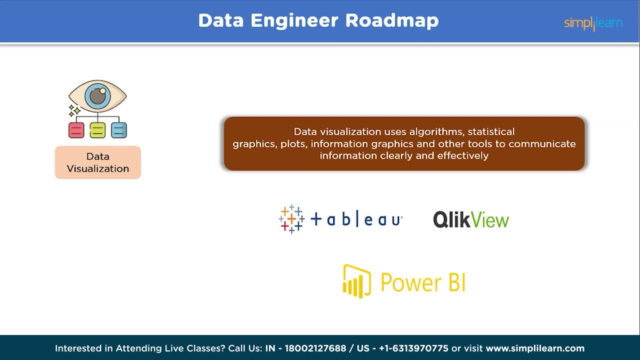 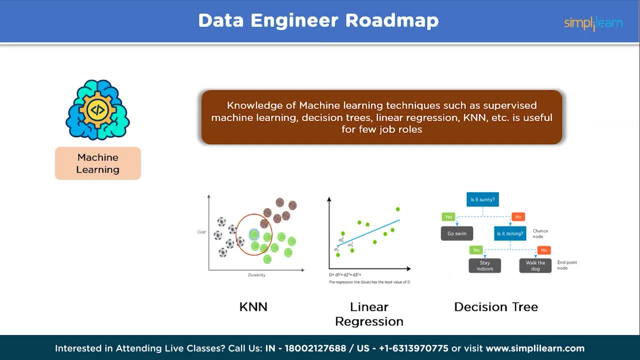 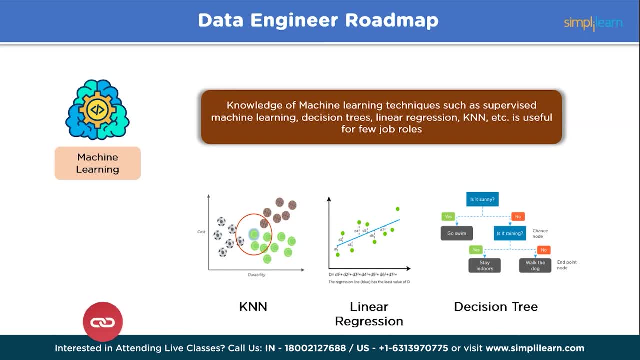 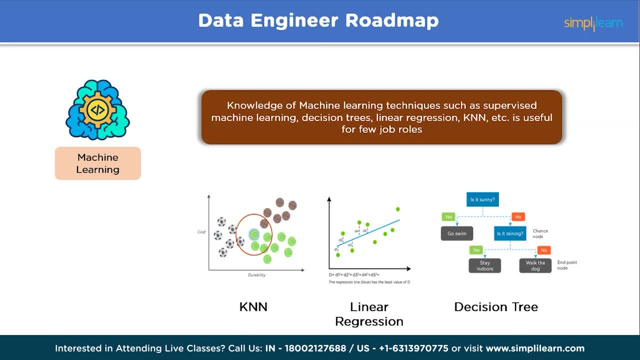 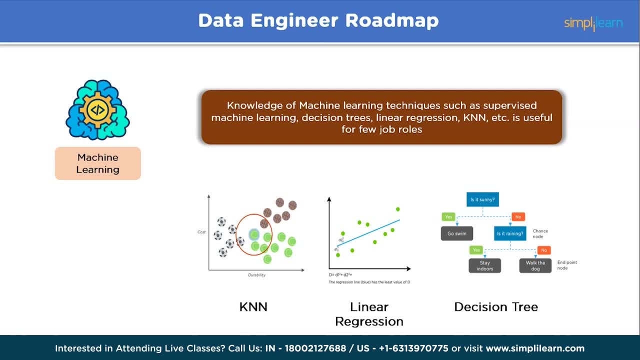 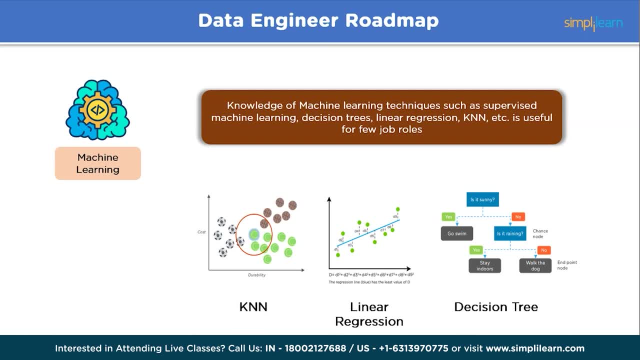 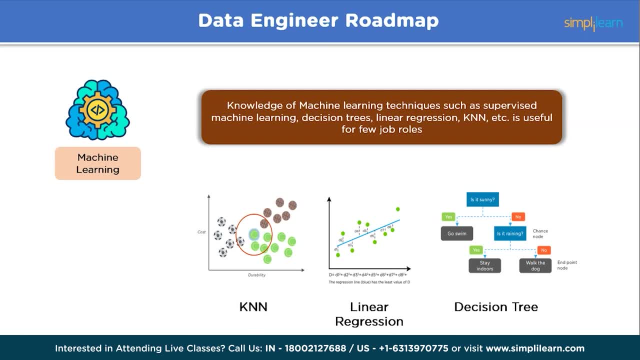 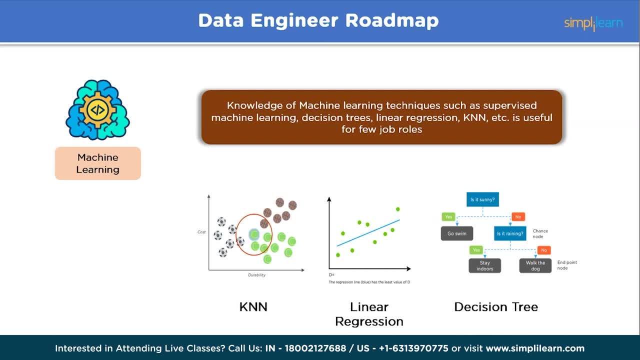 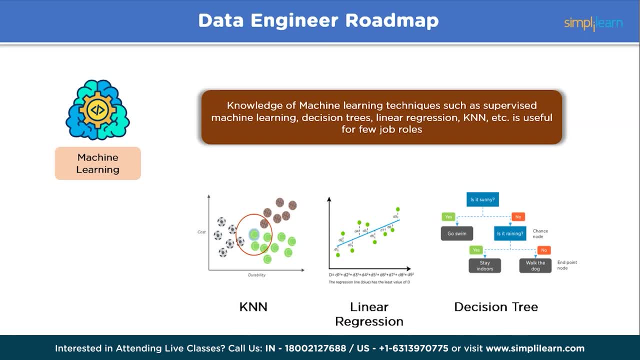 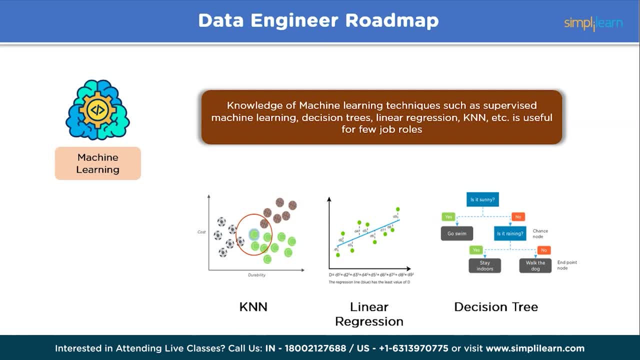 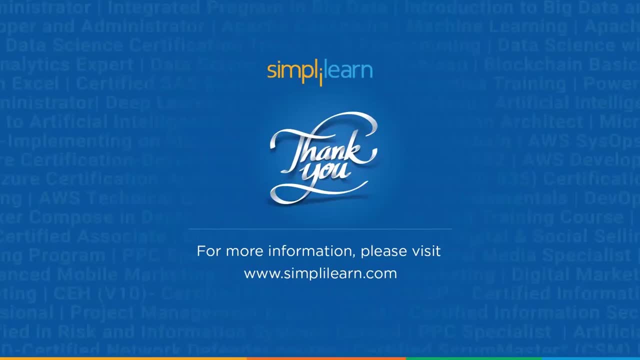 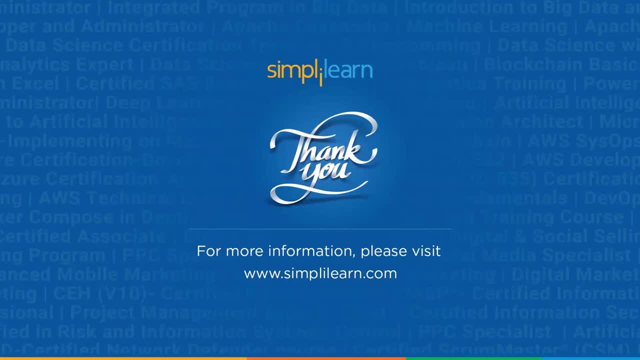 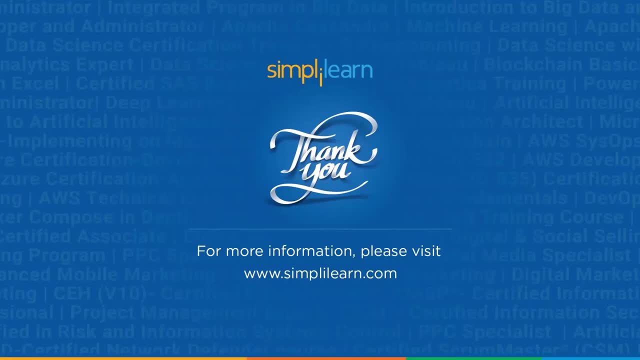 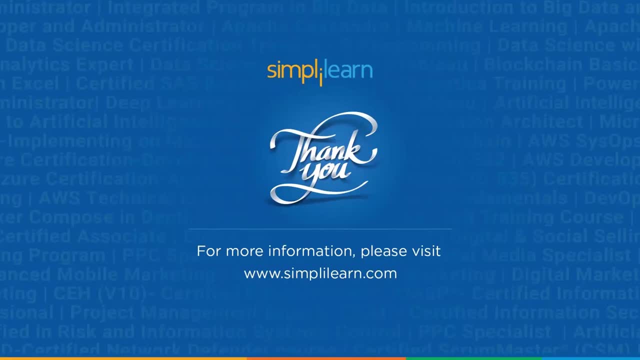 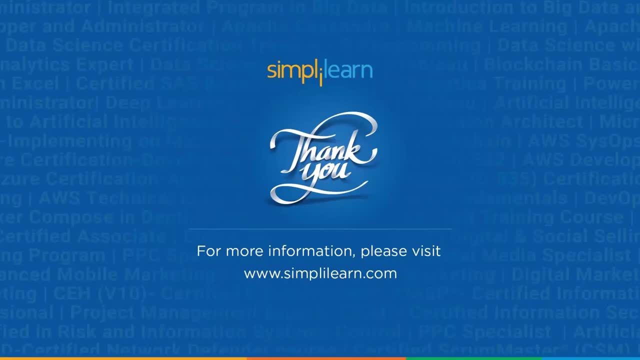 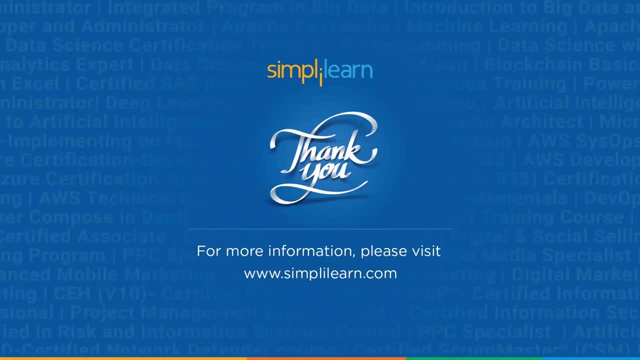 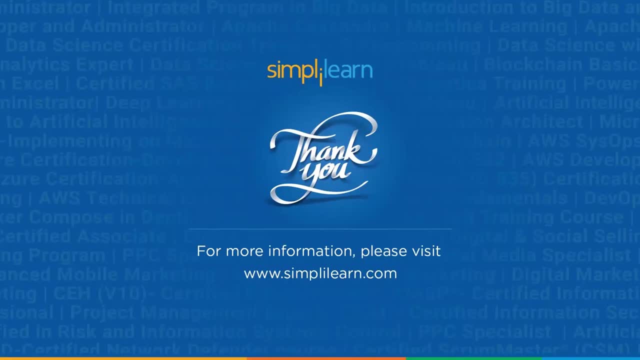 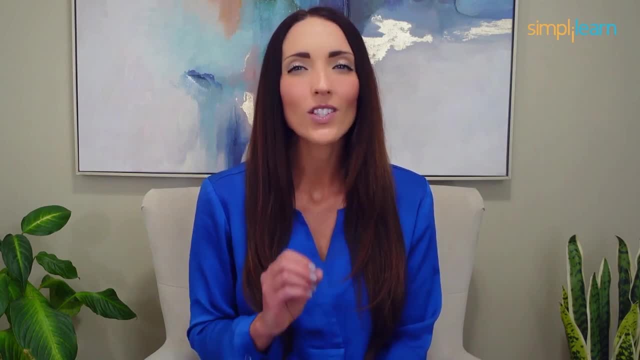 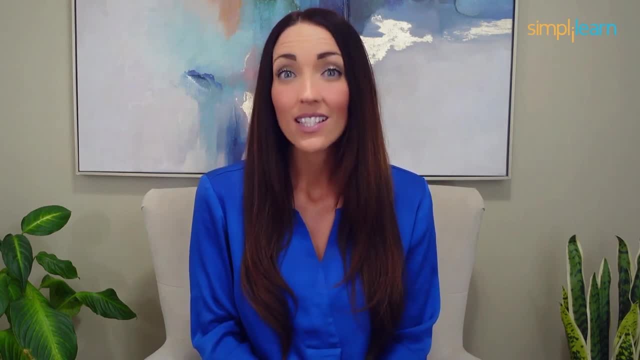 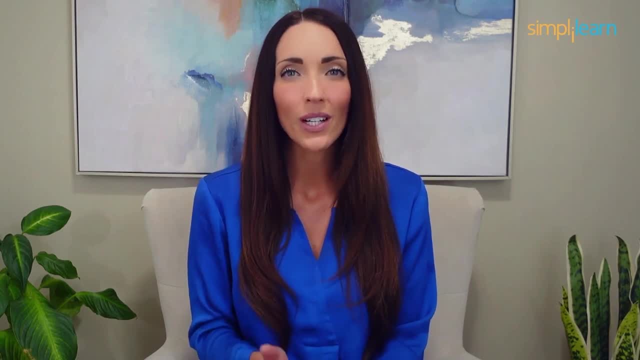 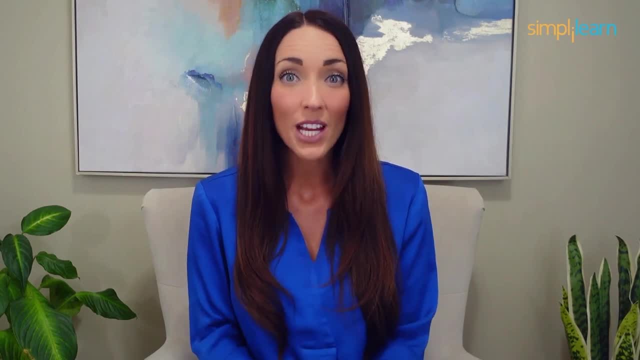 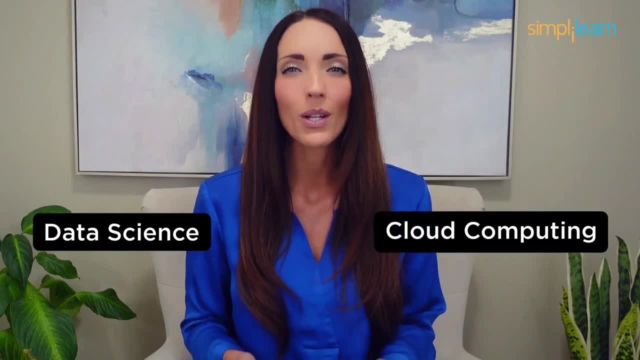